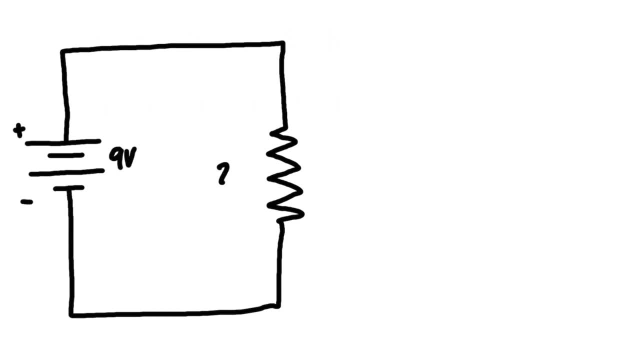 And let's say that this is a 9-volt battery with a 2-ohm resistor. So we're going to have some current flowing like this And this is conventional current, so we have current from the positive terminal around the circuit to the negative terminal. And if we wanted to, 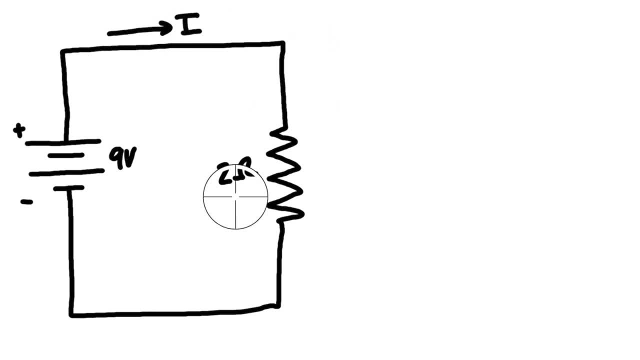 calculate the current. we would basically just want to find the total current flowing through the circuit, which is also the current flowing through this exact resistor, And we can use the expression V equals IR, which is what we refer to as Ohm's Law. Now, because there is a direct 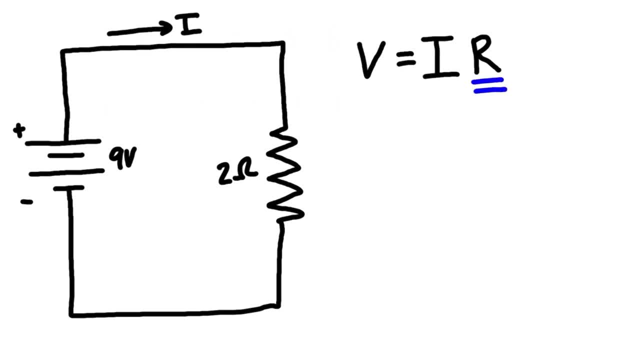 relationship here. if we were to keep resistance constant, then if we increased the current in the circuit, then we would have to also increase the voltage, or vice versa. And if we looked at it from a different perspective, let's say we kept voltage constant, then if we increased resistance in the circuit. 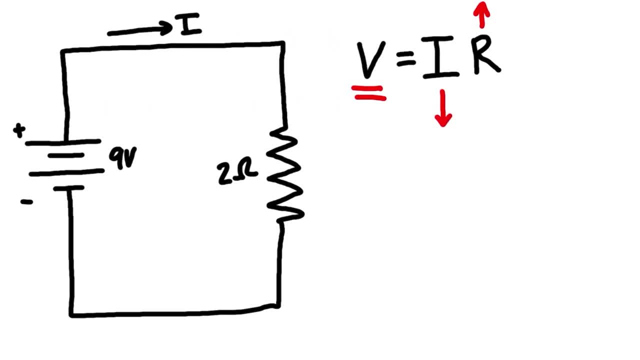 then the current would have to decrease proportionally. Now, when we look at the circuit, if we look at the positive terminal of the battery and connect the wire basically all the way up until the resistor, this is one single node And we can do the same on the bottom. 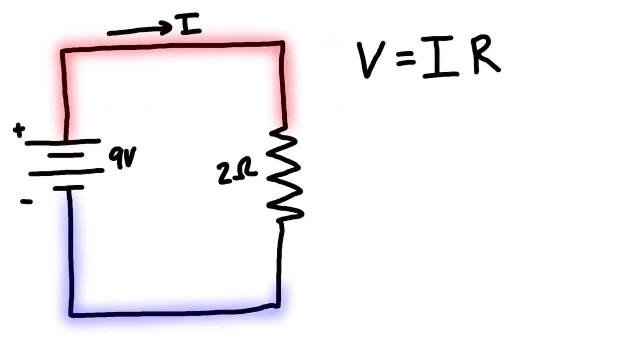 connecting from the negative terminal of the battery with the wire until we reach the element. This is another node, So everything on the blue node has a voltage. it's nine volts less than the red node, So that means that the voltage drop across the resistor. 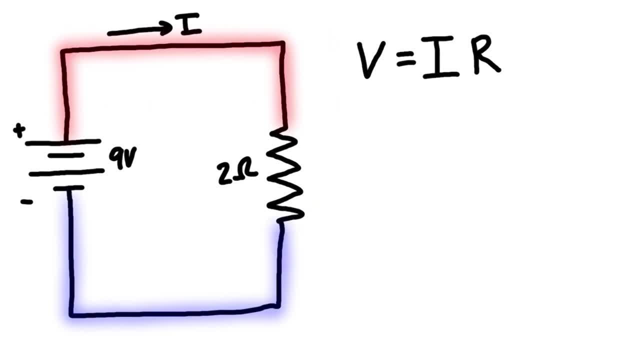 is also going to be nine volts, So we can rearrange our expression if we want to solve for the current in the circuit. we can just have. I is equal to V over R, So we have nine volts divided by two Ohms. Now the unit of voltage is volts, the unit of current is amps and the unit of 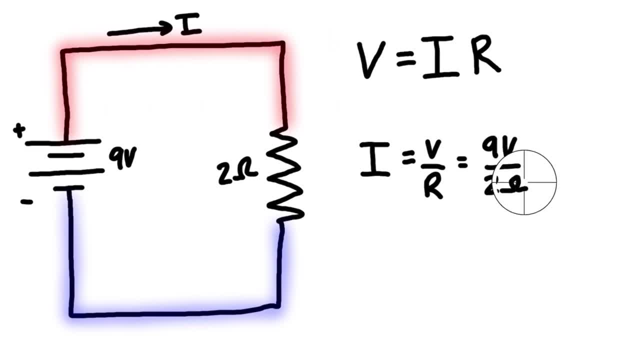 resistance is Ohms, So volts divided by ohms is going to give us amps, And we're just going to find that the current in this circuit is 4.5 amps. now let's change a value in the circuit. so let's change our resistor from 2 ohms to, let's say, 4 ohms. let's 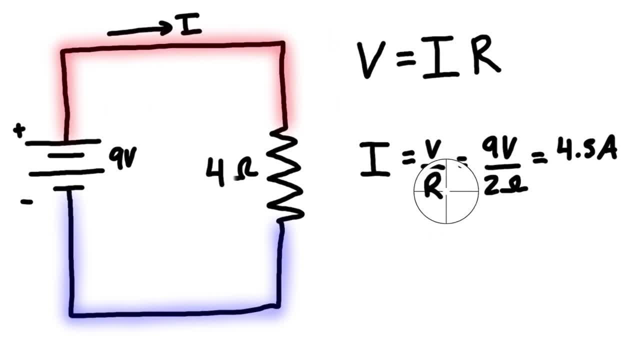 double the resistance, then what we're going to have to do is just update the value of our resistance here so we can erase that and drop in 4 ohms. and then 9 divided by 4 is 2.25 amps. all right, let's change up the values again. let's.